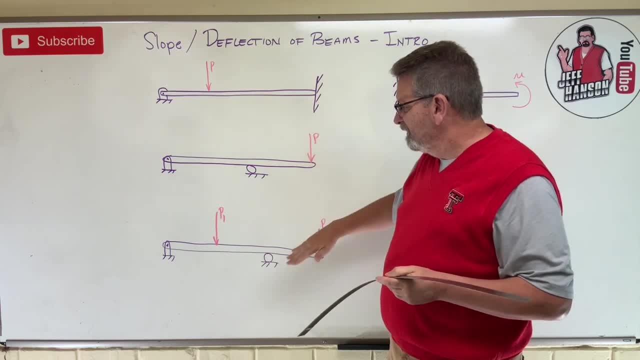 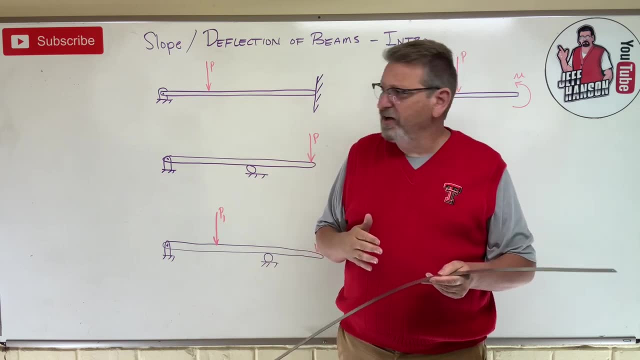 So I have drawn on the board here a couple of different beams and just with some different connections to kind of just show you how these beams are going to deflect. okay, So we're going to look, we've got one up here, that's fixed, and then pinned with a load in the middle. 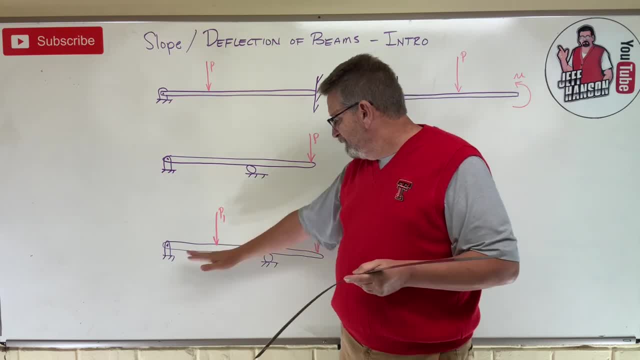 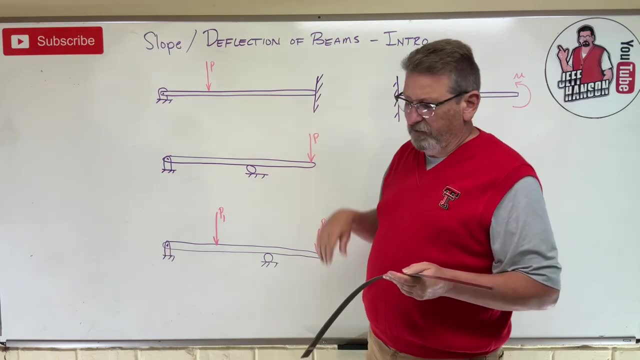 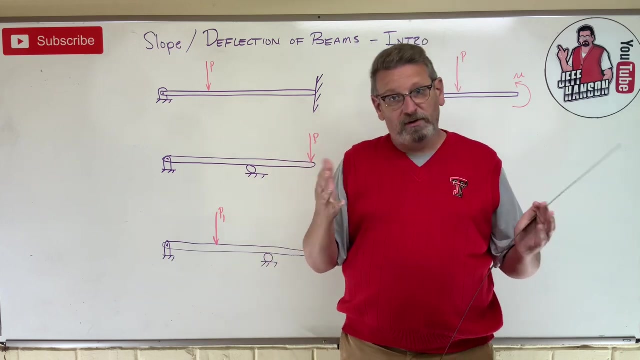 then pinned and roller, load on the end and then pinned and roller with two loads on it. okay, We're going to talk about the slope and the deflection. So first I want you just to get an idea of like, what would the slope look like if this beam had that load on it? What would it look? 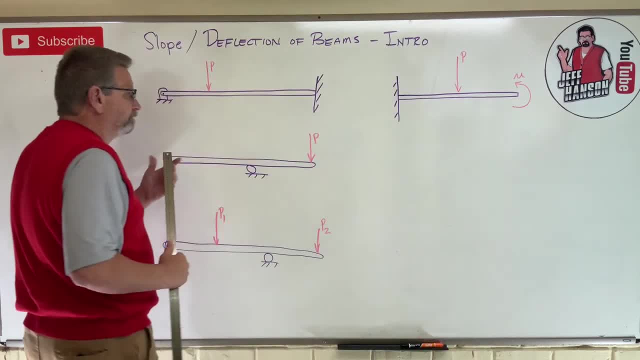 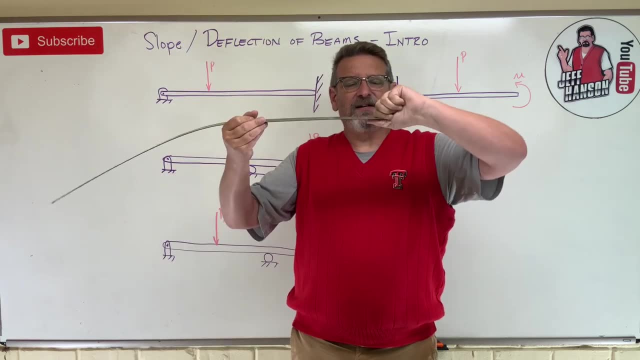 like right, So if we had this one up here now, this one has a fixed connection on the end of it. okay, So remember, a fixed connection means that it's locked, it can't move. okay, So, even if I have, 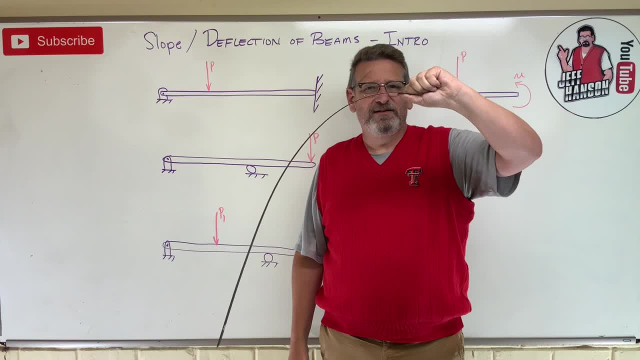 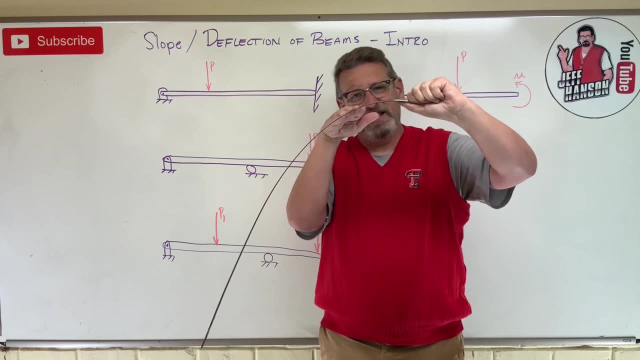 a fixed connection. now this is deflecting under its own weight. but look what's happening right at the wall. The beam is flat, there's zero deflection at the wall, and then it starts to slope right. So right at the wall, there's none. Now what if the wall was a pin connection? what? 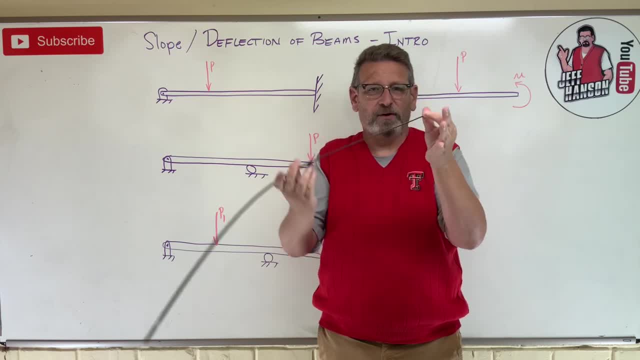 would happen. It's going to move all over the place. right, It would be like putting it on your hand and letting it swivel there, But if I hold it and I make a fixed connection now, it can't move. It's going. 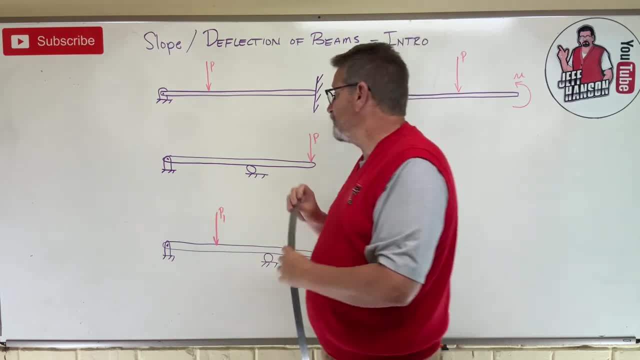 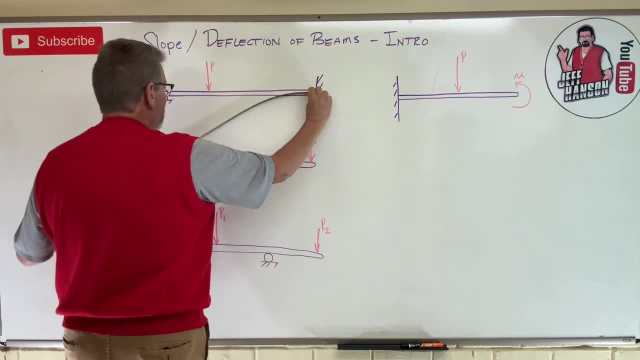 to be flat there, okay. So it's important to make that distinction. So over here we have a fixed connection at the wall, okay. Now on this side over here, we have a pin connection, and then we have a fixed connection, okay. So what is that beam going to look like? It's going to look something. 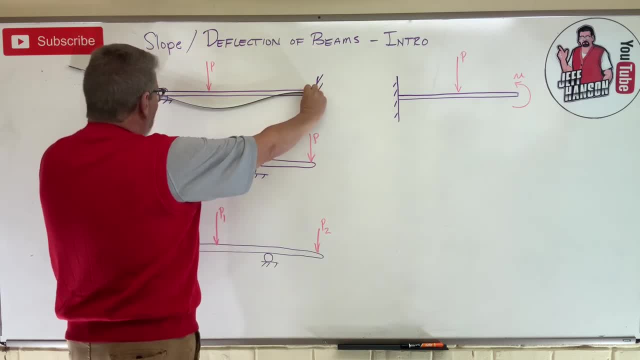 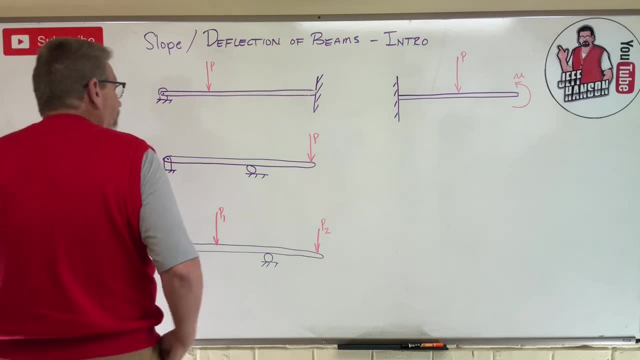 like that. So that load as it deflects is going to look just like that. Let me take this away and I'll sketch it. Okay, where's my blue sketchy marker here? Okay, here we go. So that deflection. 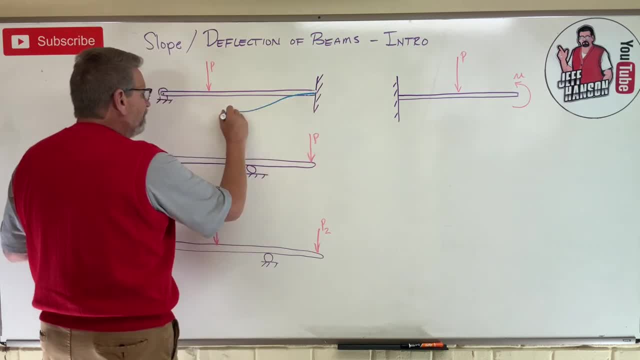 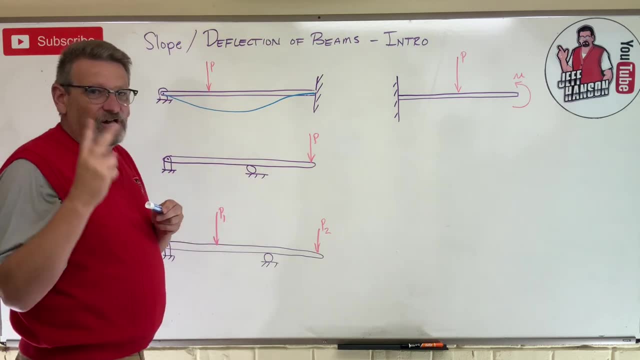 the deflected beam is going to come off the wall and deflect and come up something like that. Now, this is very exaggerated, okay, But we need to identify a couple of things here. We need to identify a couple of things on each one of these beams And the couple of things we need to. 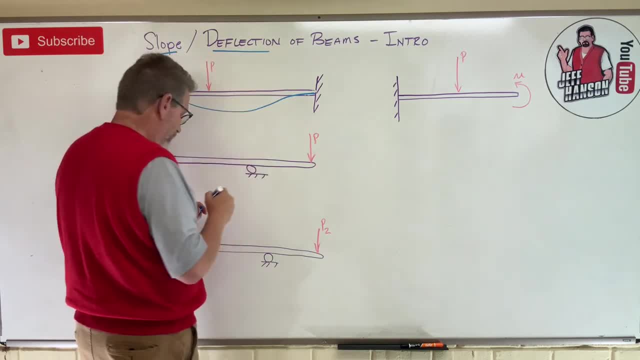 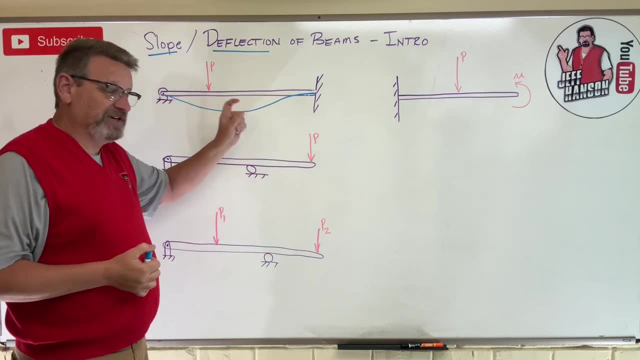 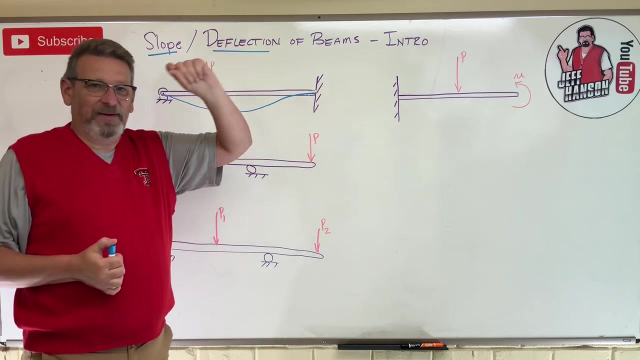 identify. are this the slope and the deflection? Because anytime we can identify, think about if I had an equation that had one of these slopes and deflection in it, if I knew what the slope and the deflection was at a point, I could maybe plug that into the equation and maybe solve for. 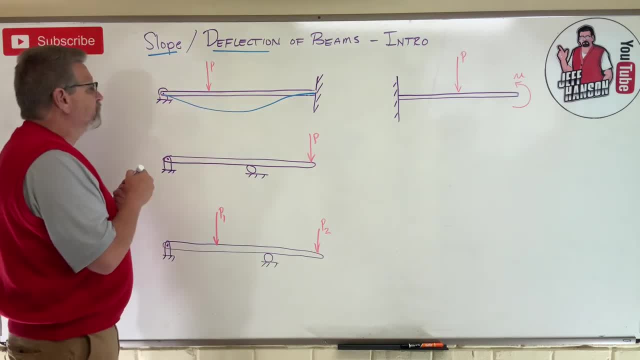 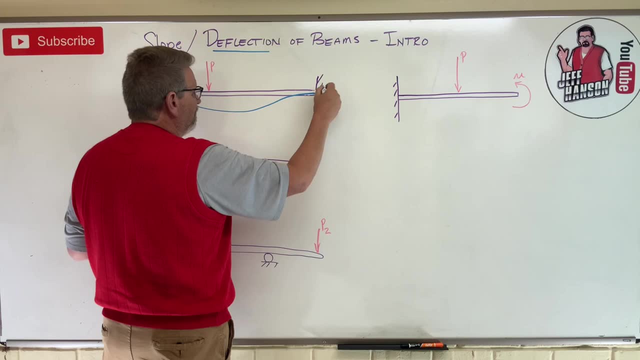 something. okay, That's exactly what we're going to do. okay. So what do we just absolutely know here? right, This beam is going to deflect, like this. Well, here's what I'm going to do. I'm going to look at this wall over here. okay, I don't know. We'll call this A and we'll call this B. 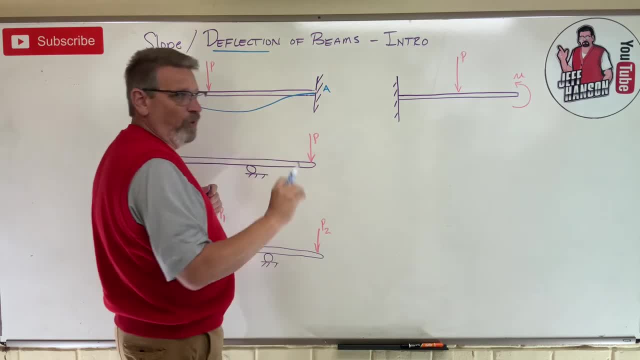 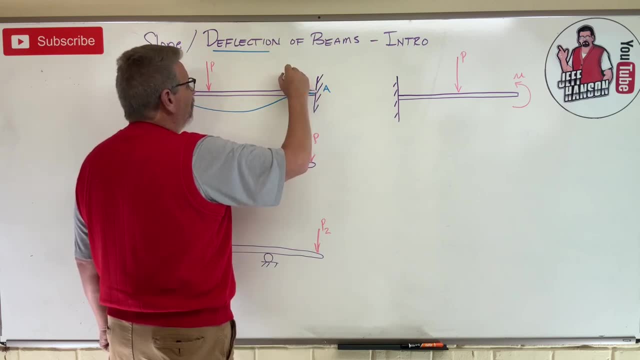 okay, At A right at the wall, right, Remember, I was holding that. What is the slope Right here? the slope, okay. Well, and I'll tell you what. Let me smear that. The slope is given by theta. okay, So it's just an angle. okay, The slope there. 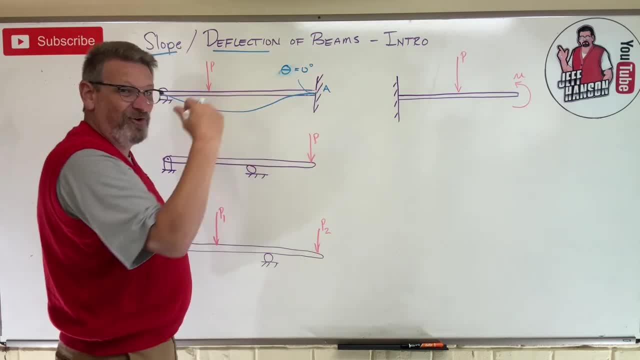 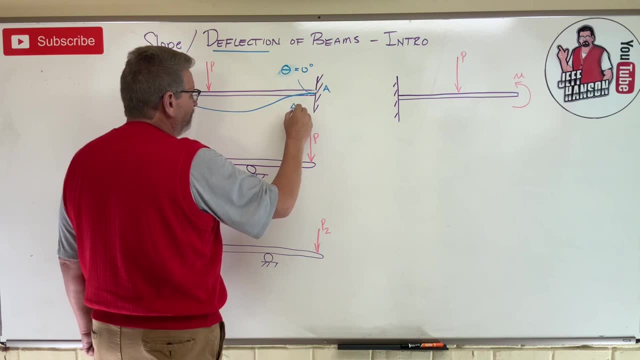 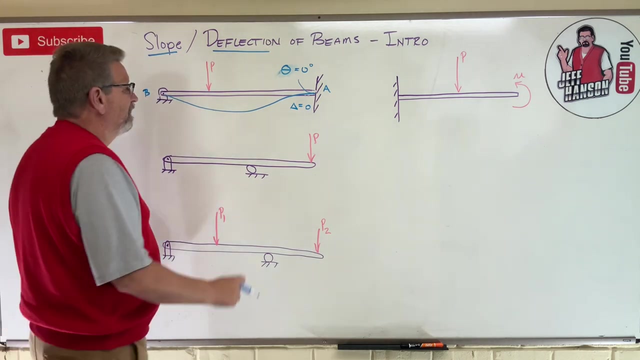 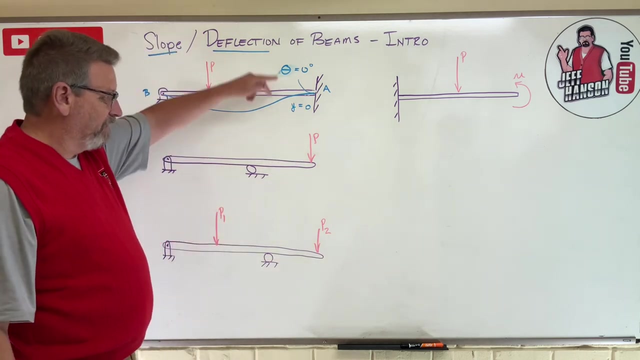 is zero degrees, right, It's completely flat right at the wall, okay. And then what else do I know? The deflection, right, The delta right at the wall is zero, okay, The deflection is zero, And typically the deflection we just call that Y, the amount of movement up and down. So at the wall, 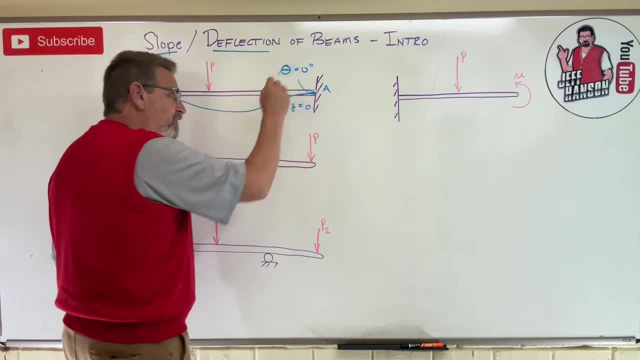 it's zero. So at this point right here, I know a couple of things, I know that the deflection is zero. I know a couple of things about that beam Now over here. I know it has deflection, I know it. 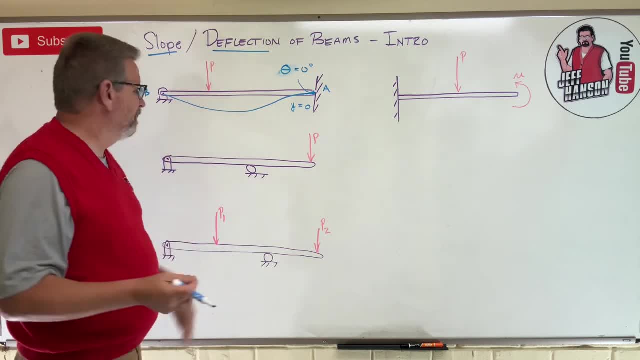 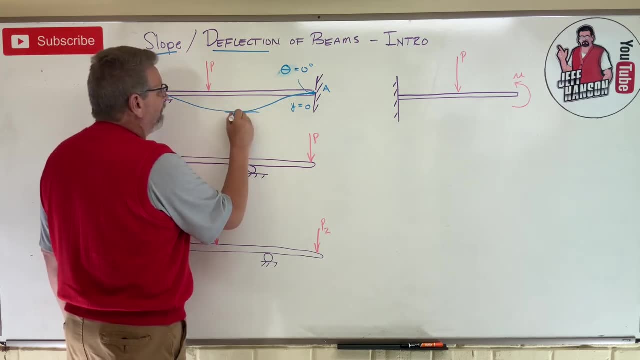 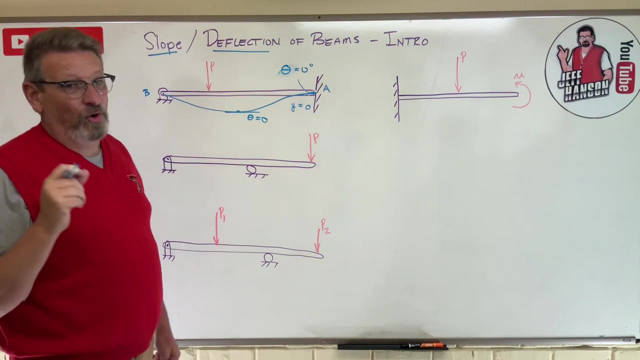 has a slope. I got no idea what it is, though, But at some point I go from being going downhill to start going back uphill, And at that point, right there- guess what? The slope is equal to zero. Now the problem is, I may or may not know where that point is. okay, Some of the things. 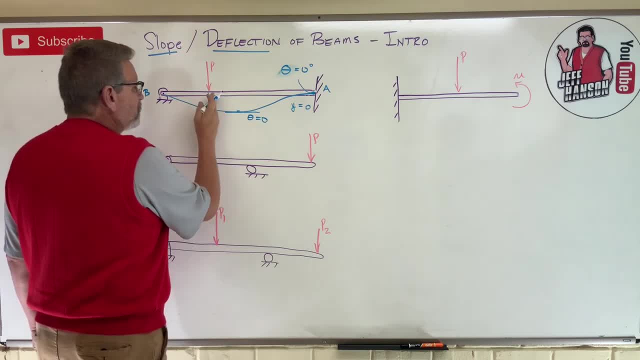 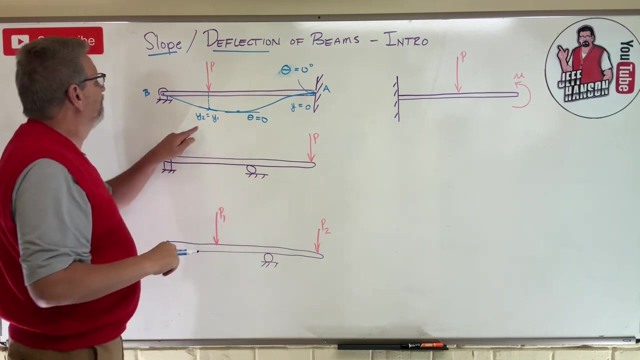 that I know, if I get over here at this point, I know that the deflection is zero, I know that there's a slope on that side of that line. There is a slope there And the slope on the other side, right, Right, at that point, this Y- we'll call it Y1, is equal to this Y, right The slope. 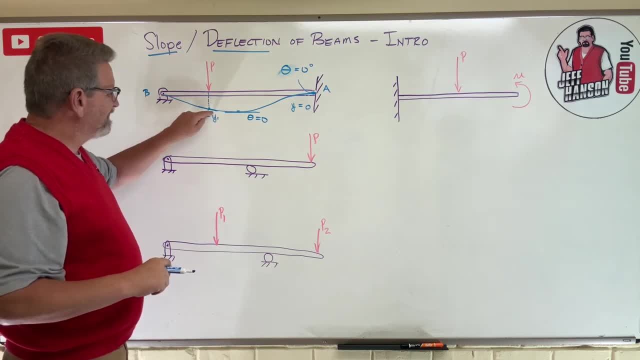 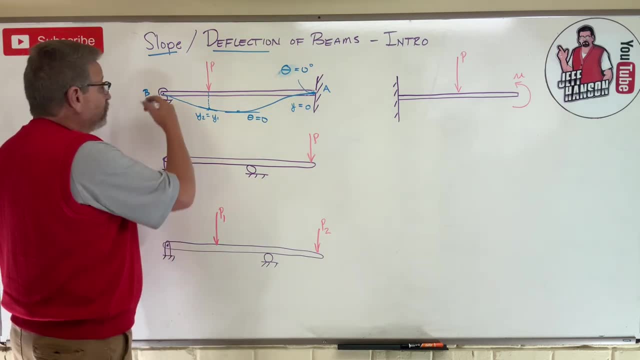 just one molecule on that side of the dot is the same as the slope, as one molecule on that side of the dot right. And then over here at B. what do I know? Do I know the slope at a pin? There is slope, but I don't have any idea what it is. But here's what I do know. At this pin over, 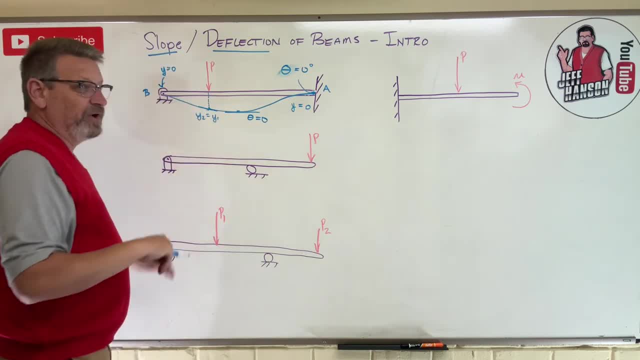 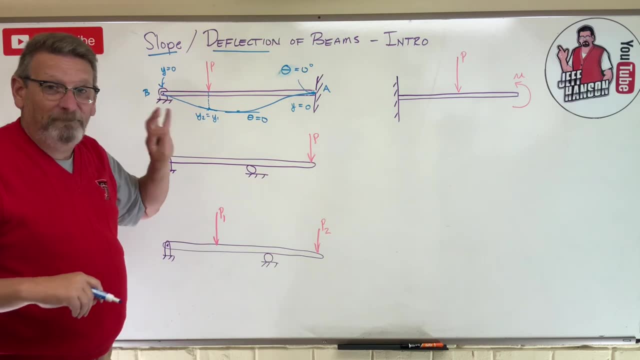 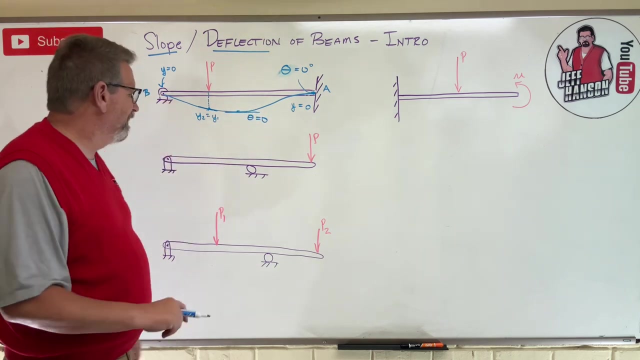 here, Y has to be equal to zero. There is no deflection because it's got to come back up to that pin right. So those things which are called our boundary conditions, you know, being able to identify these things just using logic, just using your head, super-duper important okay. 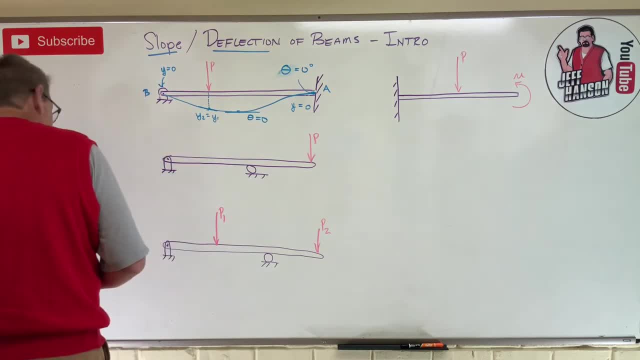 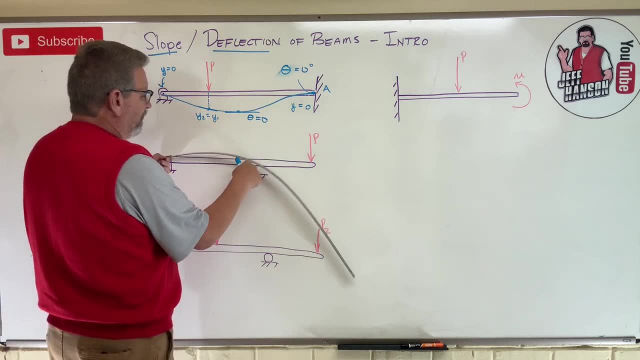 What does this guy look like? I don't know Where's my B. okay, I'm pinned here, right, But what do I have over here? I'm going to use just my finger as the roller connection. I'm pinned here and I have a roller there, and then I have 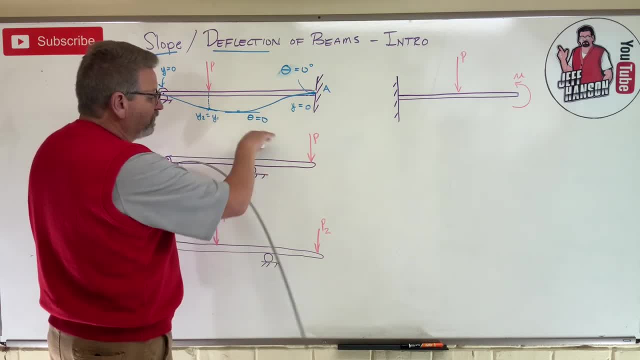 the load over there. What's it doing? The load is just pushing it down right. But look, between the pin and the roller, what's happening? It's kind of humped up a little bit, isn't it right? So what does that beam look like? That beam kind of looks like this: 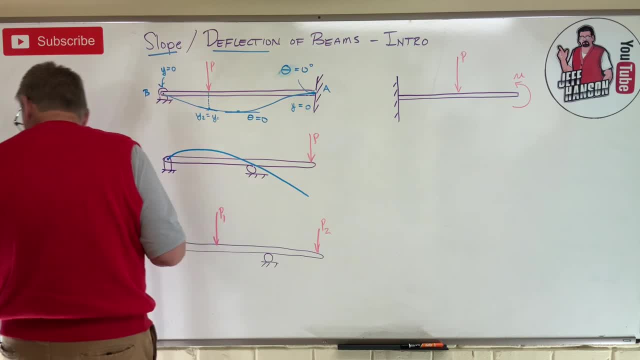 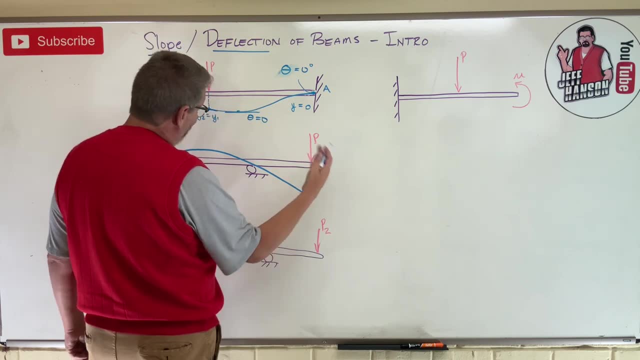 Okay. So again, what do I know about this guy Over here? I know there is deflection, I know there is slope. I got no idea what it is, though. right. But right there, what do I know It has? 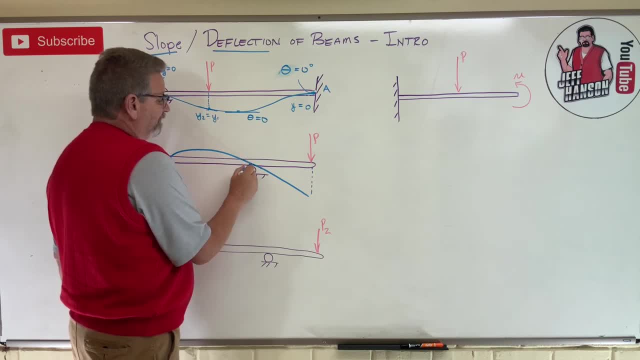 slope. Again, this side of the thing and that side of the thing, the dot right, The slope Y1 has to equal What That's not slope, That's not slope. It wasn't slope either, was it? Why did you put Y for slope? No, that's theta. Sorry, Theta 1,. 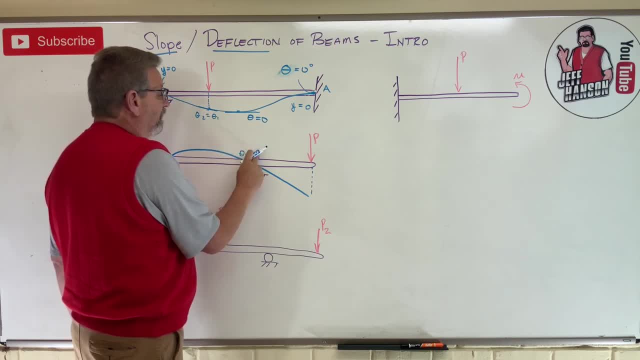 theta 2, right. So here theta 1 equals theta 2, okay. What do we know about the deflection at that point? Well, the deflection is Y and at that roller it has to equal 0. Again. 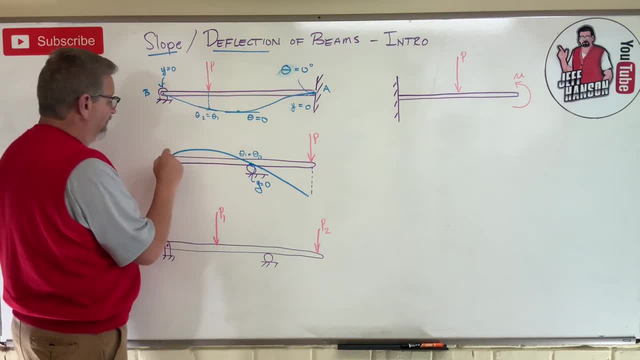 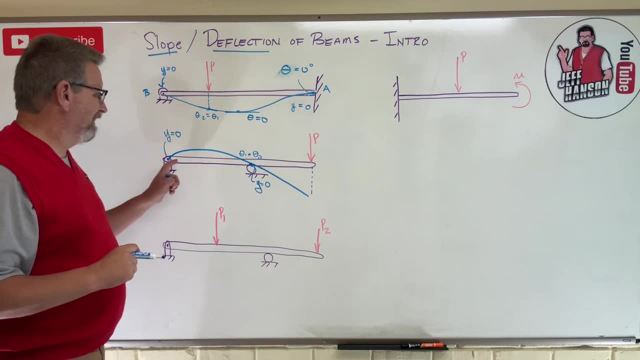 what about over here? Well, it's got slope. I don't know what it is, but I do know that Y has to be equal to 0.. There is no, No deflection at that pin. Are you kind of catching on? This is just kind of logic stuff. 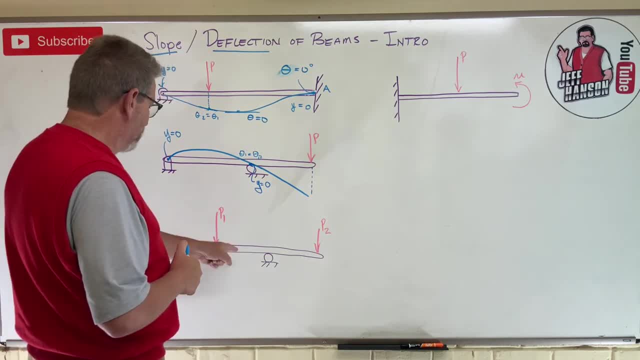 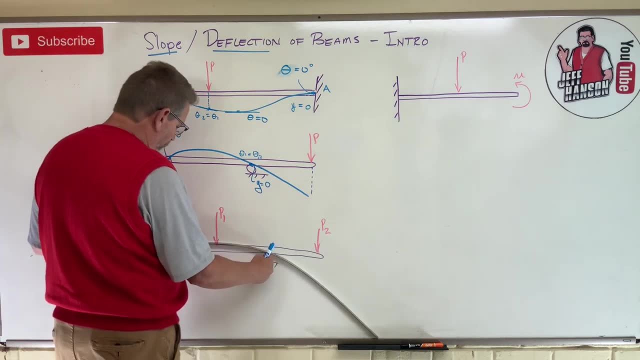 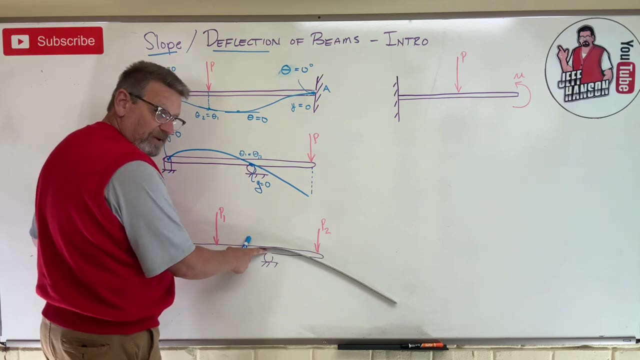 isn't it? Now, what in the world is that one going to look like? Well, let's see, Because now what, We're pinned over here and we're roller over here, okay, But we got a force in the middle, So we're kind of going to be a little bit of an S-curve, Do you see that? It? 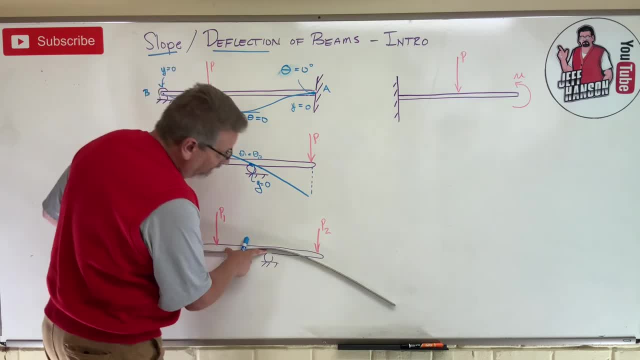 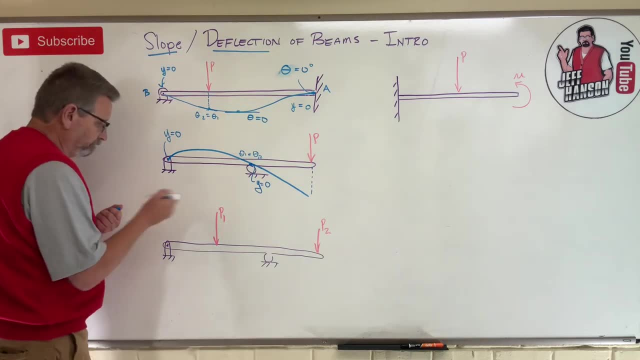 goes down, goes back up to the roller and then, on that end, back down again, doesn't it Okay? So what's that going to look like? Kind of like this Down and then back up and then back down again. okay, Well, that's kind of. 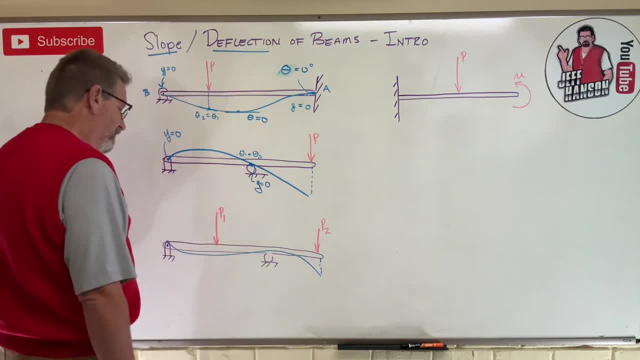 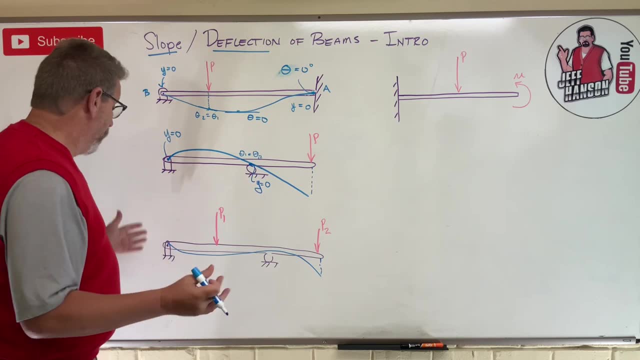 All of this is very exaggerated, right. I mean, who's going to build a beam out of the world's flimsiest ruler? I mean, we're not doing that, right? Okay, So again, what do I know? Okay, 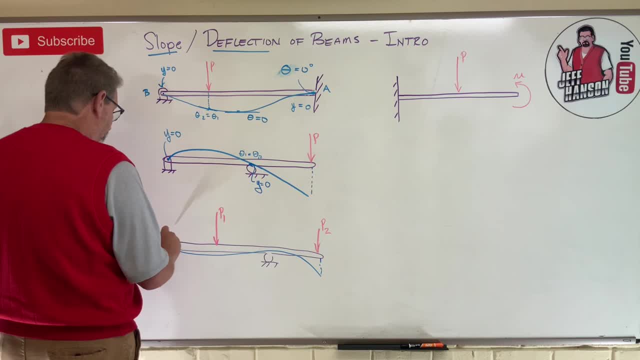 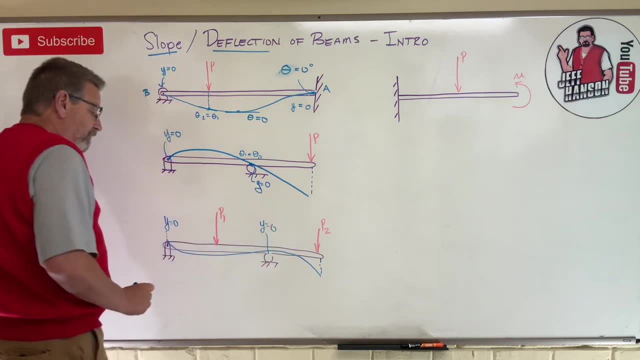 Here's what I know. At this point, right here, there's no deflection, so y equals zero. At this point, right here, there's no deflection. y equals zero, right? Do I know anything about slope? I know that it's zero somewhere over here. 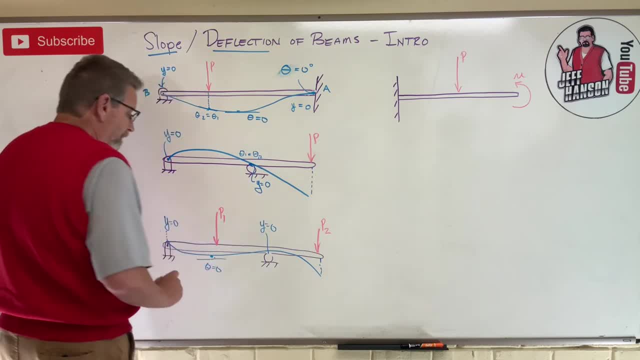 right Slope is zero, But do I know where it is? Is it necessarily right under that force, right there? Well, if that force was exactly in between these two forces, or these two points rather, and it was completely symmetric, I'd say yeah. 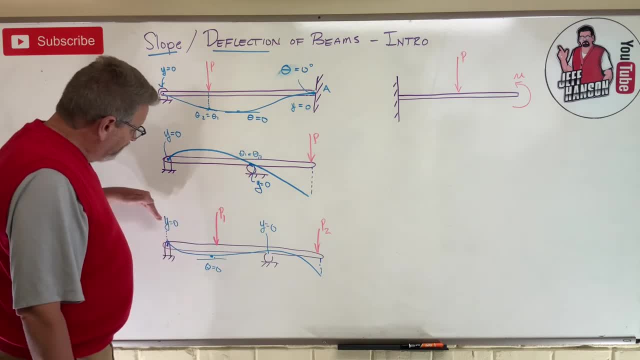 Probably. But if it was more to this side, the force may actually keep on going down past the force and then come back up. So I can't really say where that's zero, but I do know that the deflection there is zero and the deflection there is zero. okay, I don't know what it is over there. 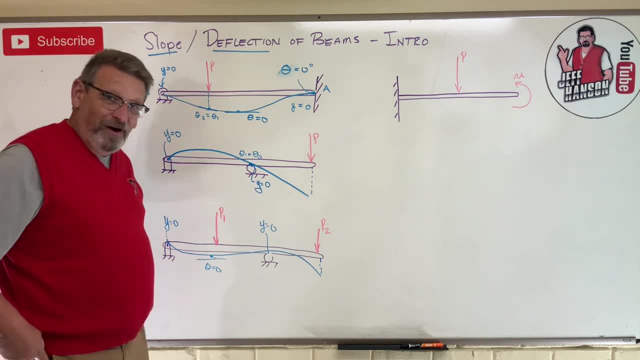 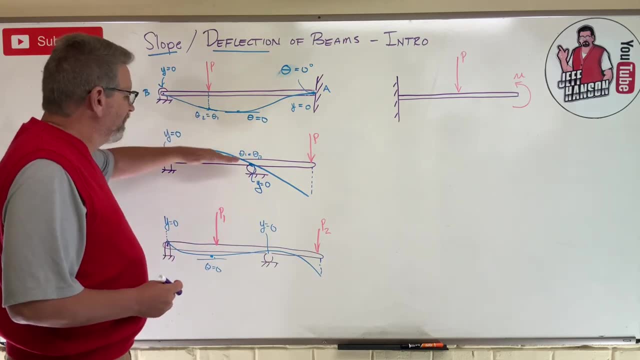 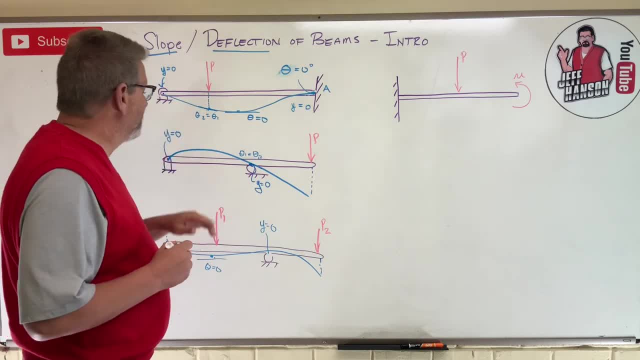 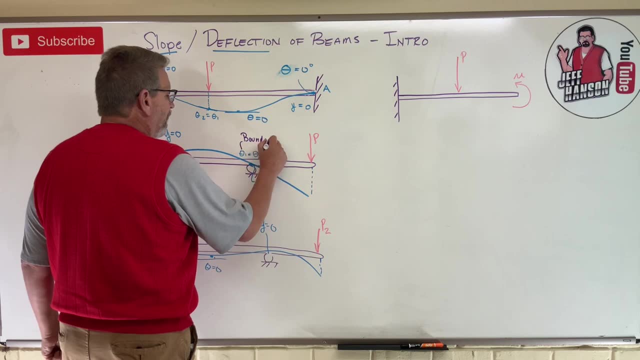 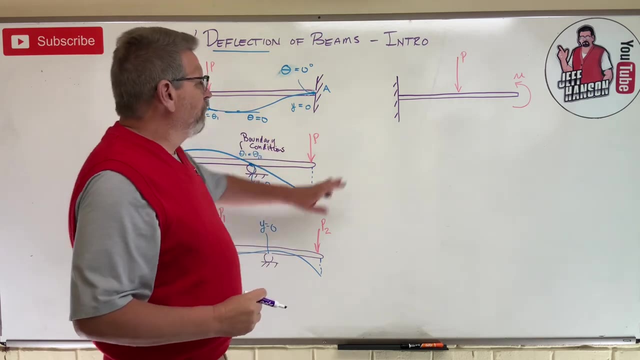 Some of those deflections kind of look like the slope and deflection, And again, these things are called our boundary conditions. okay, Boundary conditions, Okay. Let's look at one more, And what I have over here is just a beam. And what I'm going to do, 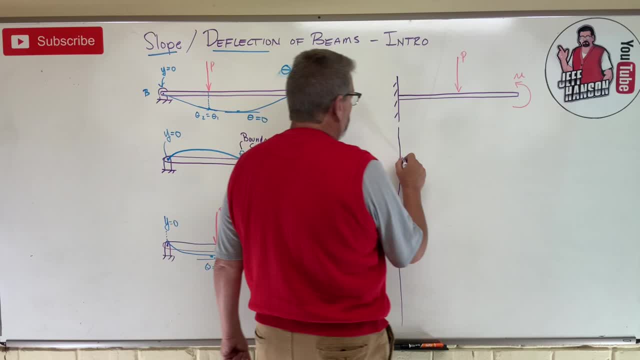 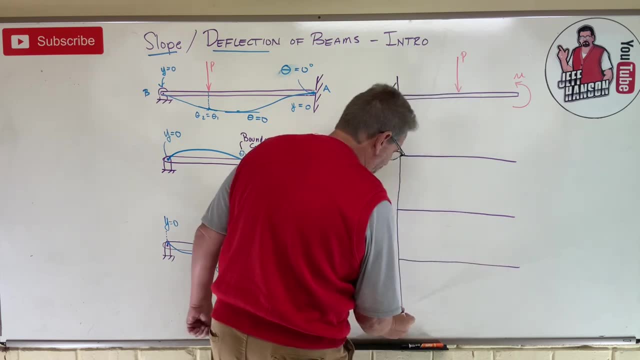 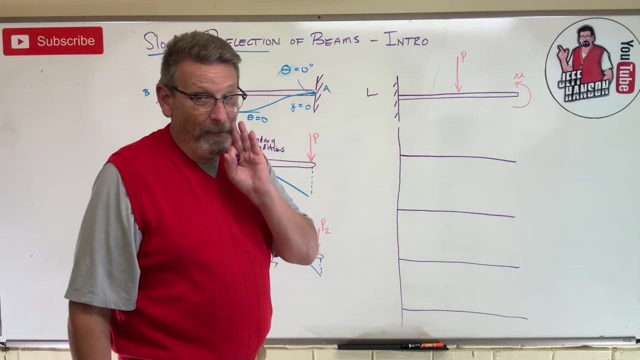 for you is. I'm going to show you. here's what we're getting into. okay, Here's what we're getting into. What is he doing? Okay, We've done this before. We call this L for load curve- Sure moment diagrams. Sure moment diagrams. Okay, Here was the V curve, right, This? 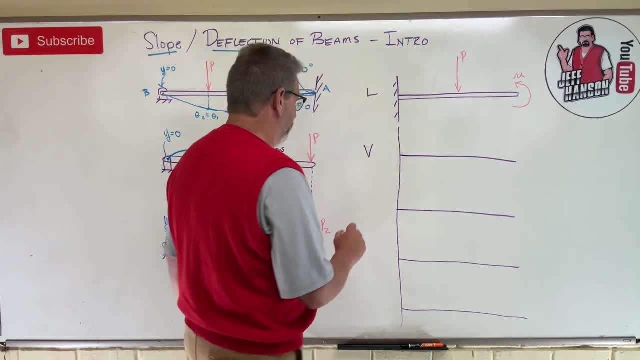 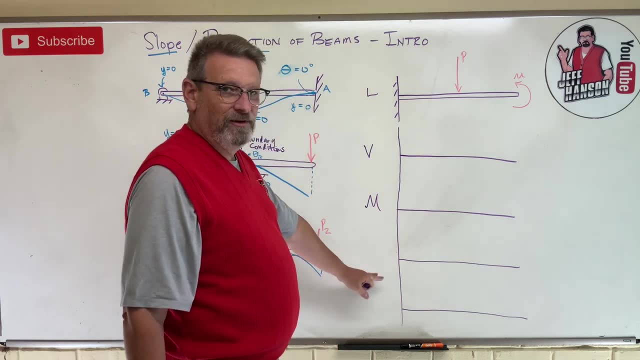 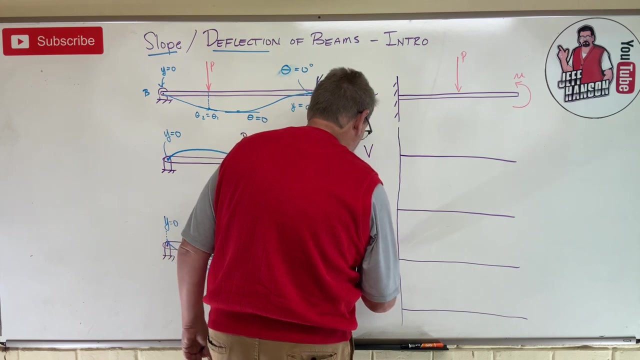 this was the integral of that. What is the integral of this? Well, that was the bending moment: curve. Why did you draw two more, though? Because I can integrate this one and get the next thing, which is the slope. Okay, The integral of the M diagram gives: 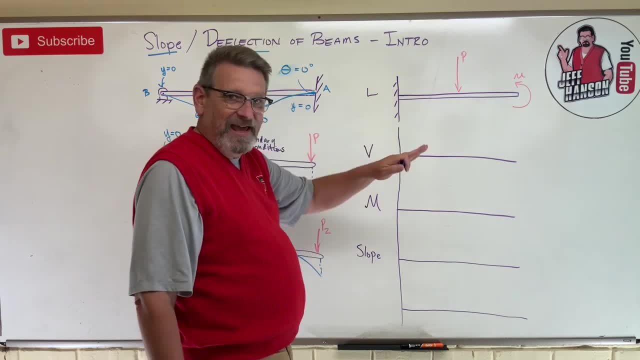 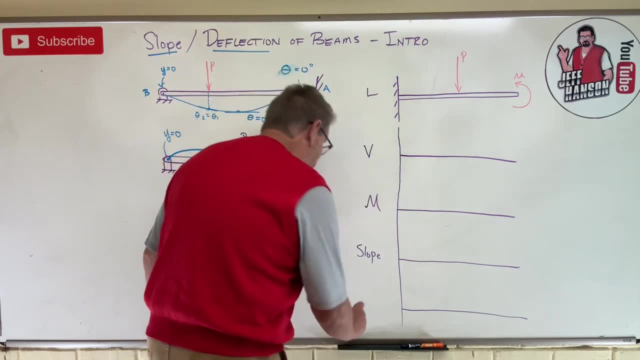 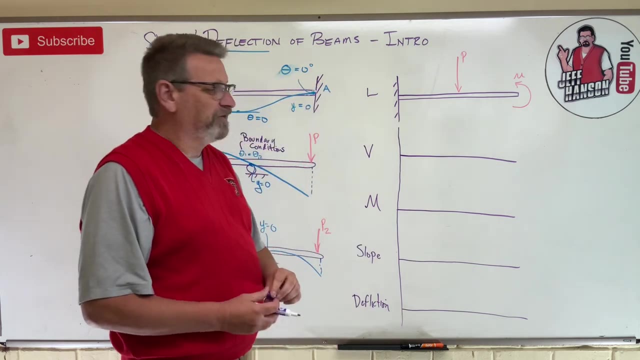 me the slope. I can tell you the angle of the beam at any point along its length. What Then? I can integrate the slope one more time. Okay, Okay, And I get the deflection of the beam. How much is it from there to there? How much is it from? 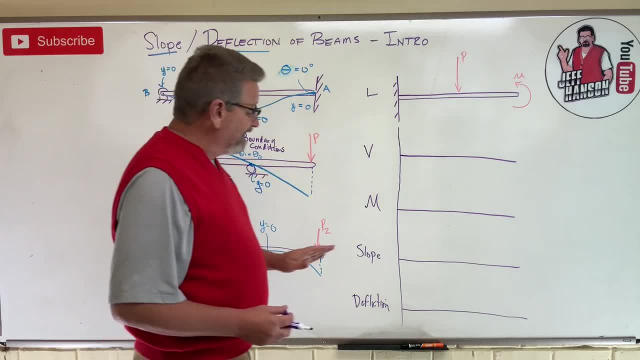 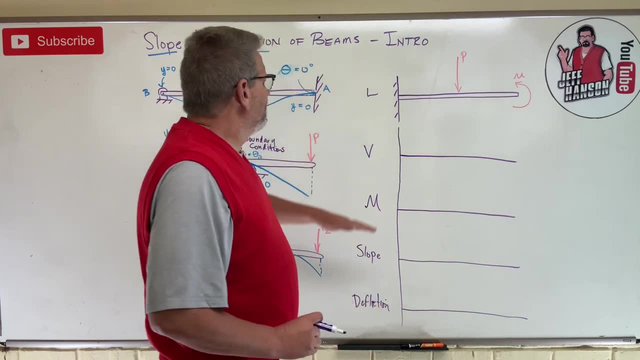 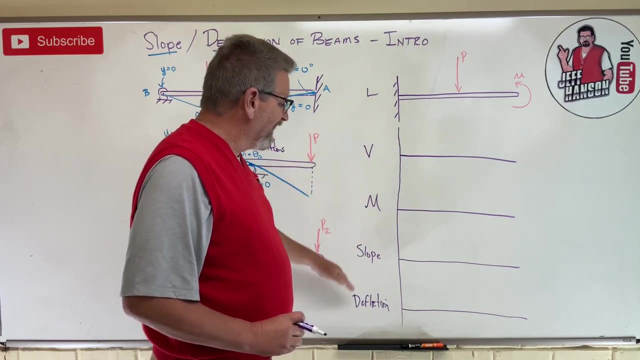 there to there. What about over there to there, right? I'm going to be able to calculate that with some equations. That's an E right there, by the way, deflection okay. So one, two, three, four, five things I can integrate four times to get down to there. It's going to take a lot of. 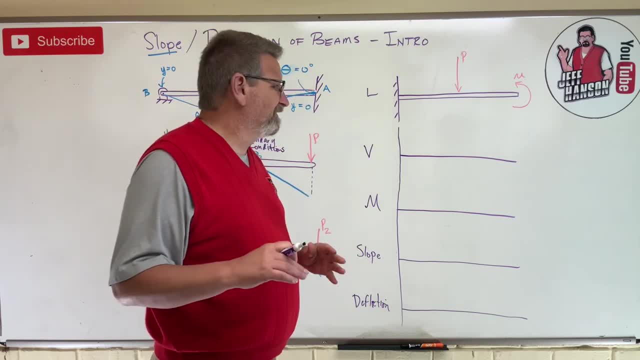 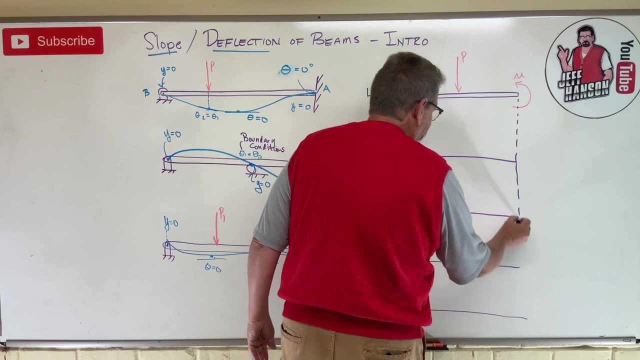 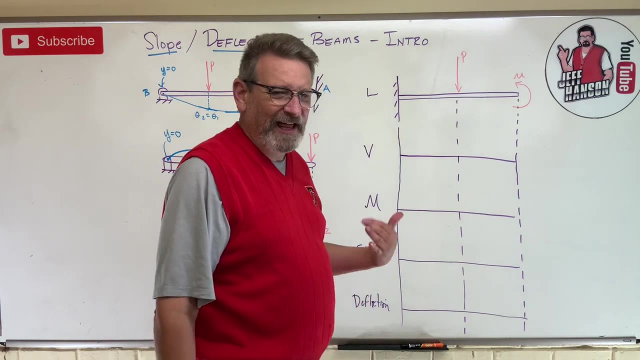 math y'all, but it's not super hard, but it's going to take a lot of brain power. but I got you. okay, Here we go. Let me do this for you. okay, Can we plot this? No, you only have letters Come. 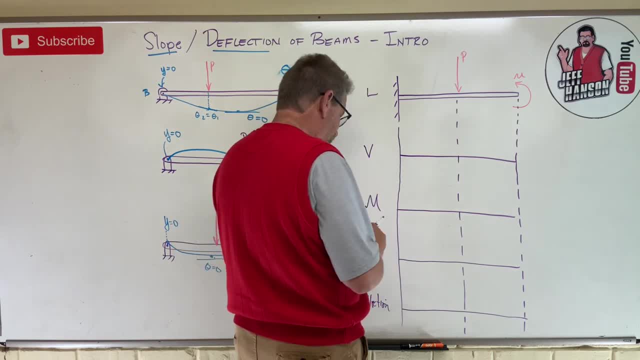 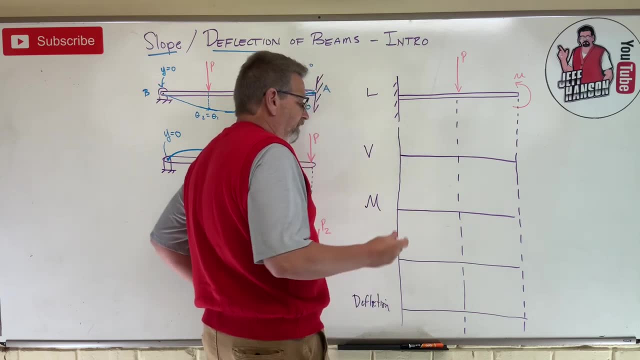 on man. Come on man, Let's try it. Where'd my blue marker go? All right, let me see here. Let's see if we can do this. Here's my blue marker. okay, Global equilibrium. up here, you know. 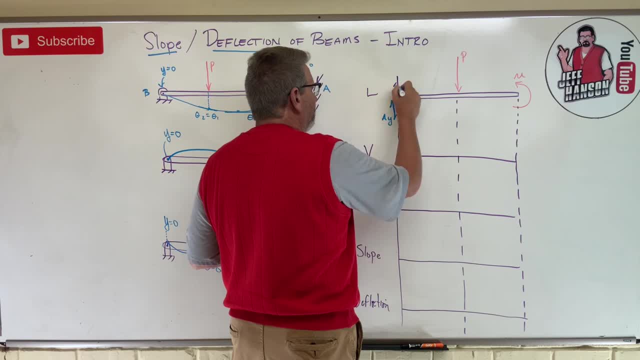 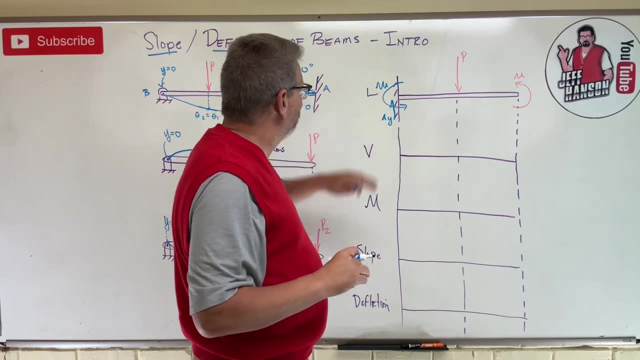 I've got what? I've got an AY, and then maybe I have this right- An MA. I got an AX, but he's zero. okay, So I've got this right. So can we graph this? And what I'm just worried about here is: what does the shape look like? 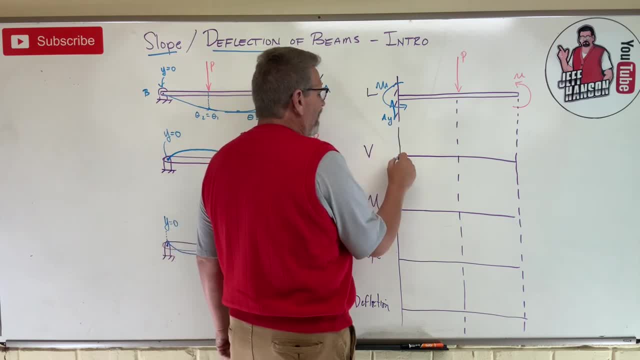 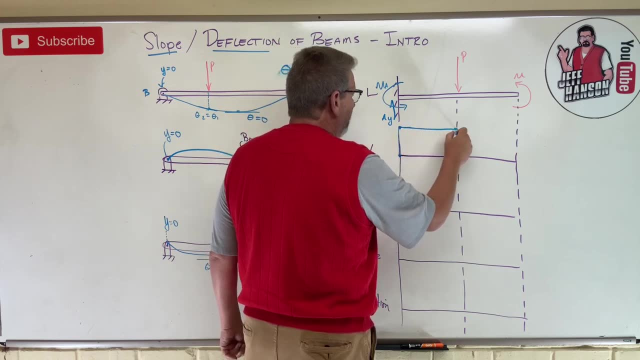 right, The V diagram. okay, Boom. AY, Van Halen force Might as well. oh jump, okay, No change, no change, no change, bam what P goes down whoop and then zero all the way out, right? 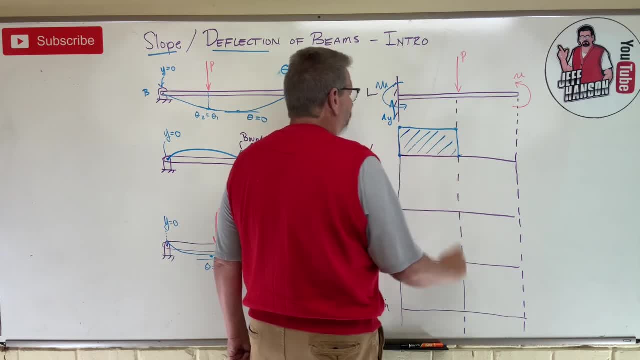 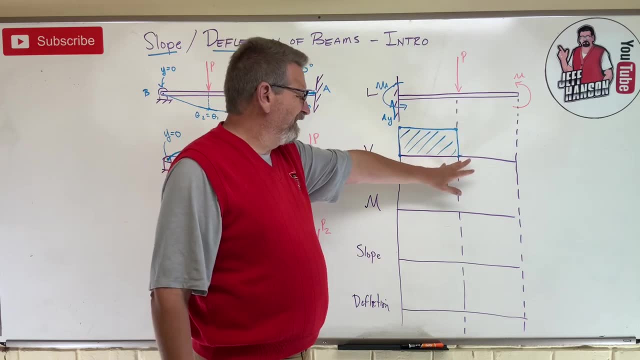 This is what our V diagram looks like. okay, We have shear from here to here, no shear out there, and then that bending moment on there doesn't affect this diagram, but I bet it affects this one, don't you think? okay, Let's go down to the next one. What do you? 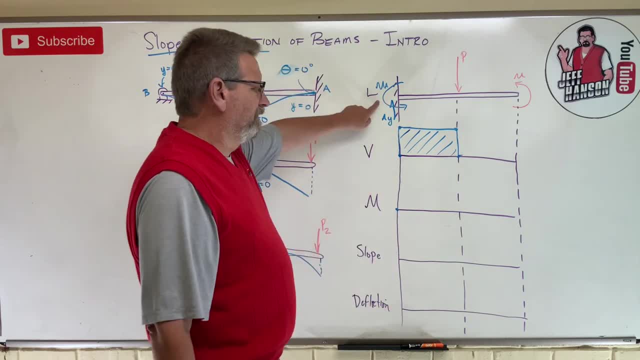 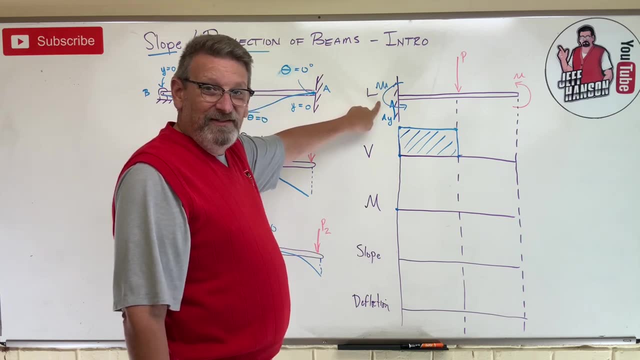 get. You get down here. okay. We start off with a kitchen force. Remember this guy. a moment. In the kitchen, the clock is above and the counter is below, and let's go down to the next one. We start off with a kitchen force. Remember this guy. 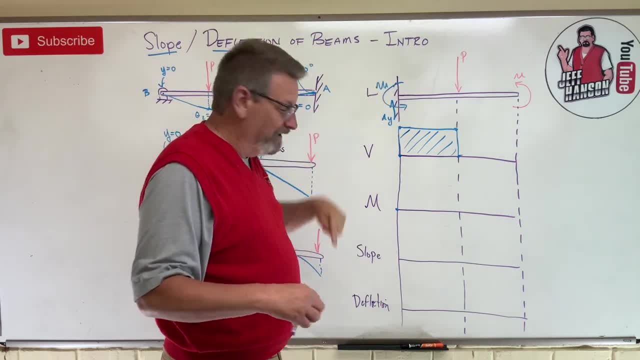 a moment. In the kitchen, the clock is above and the counter is below, and let's go down to the next one. Let's see what this is. That's counterclockwise. so it's going to make us go down, isn't it? 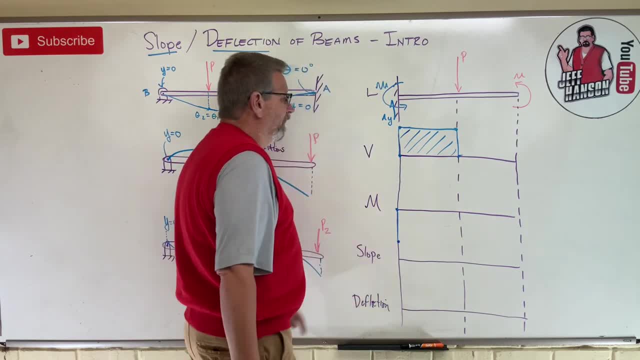 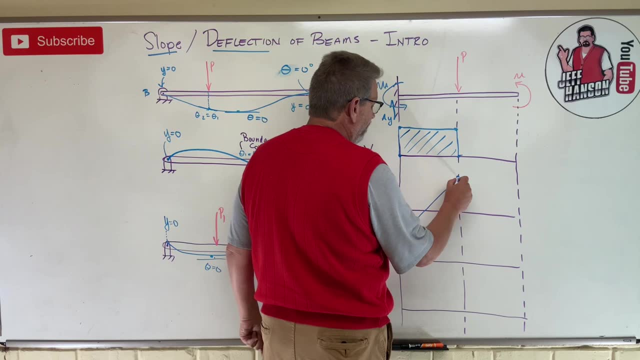 So here we go, whoop, and then what? I'm going to come up, some from this shape here, okay, So up, okay. And then from here to here. how much moment was there over there? None, so no change. 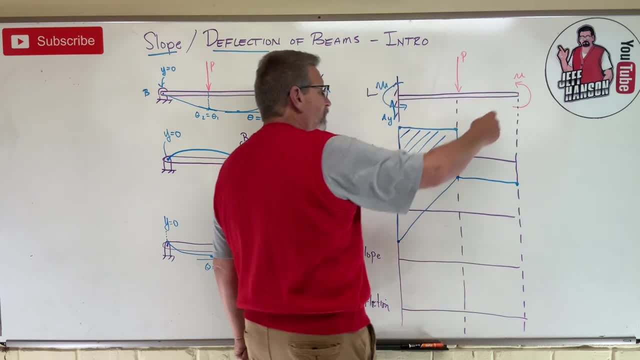 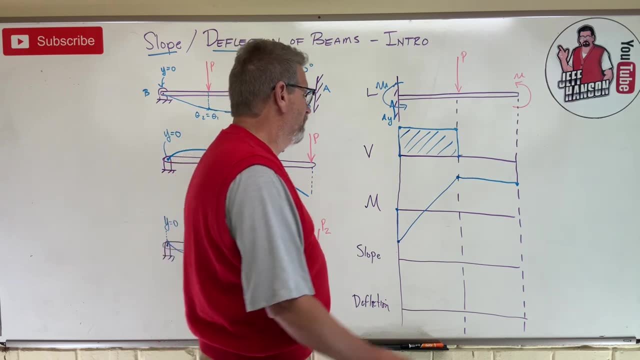 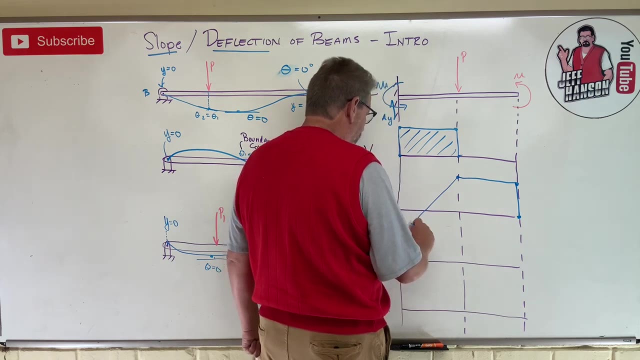 no change, no change. and then what? What do I have over there? Another concentrated moment, and that guy is a counter below right, So it's going to drop me down. take me home to the place I belong on my moment graph. 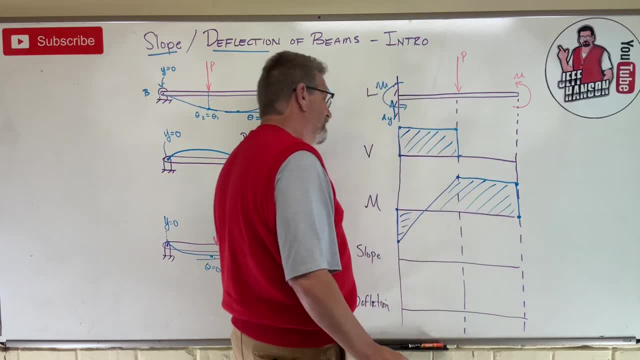 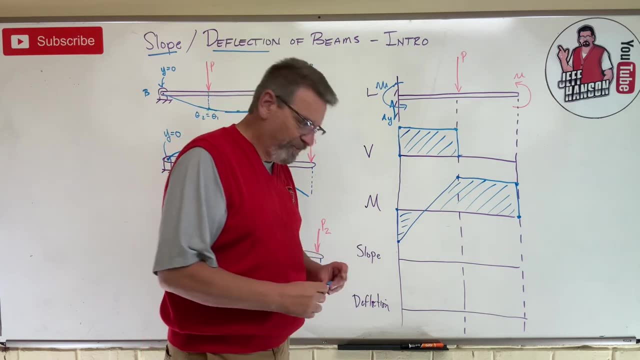 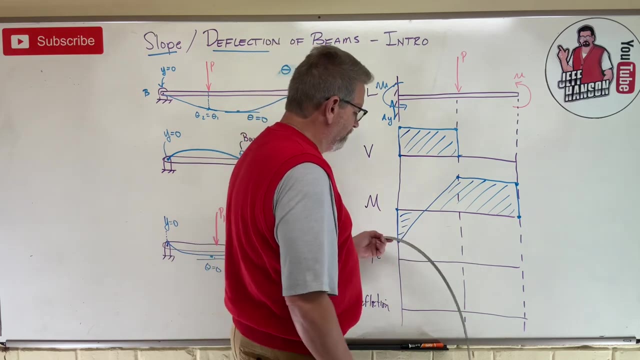 back to zero. okay, And there you go, and that would be your moment graph. That would be what that looks like. So what about the slope? okay, Let's see if we can kind of think about that for a second. What would the slope of this guy look like? okay, Because what we got here is I've got. 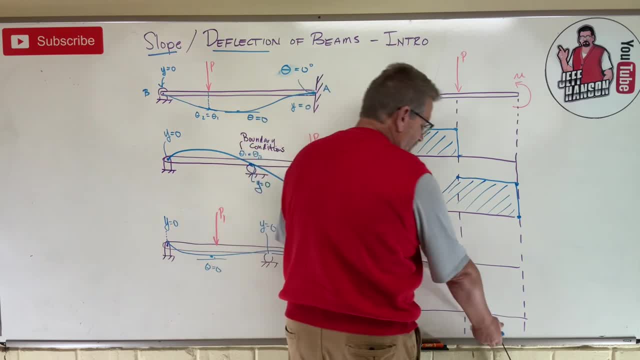 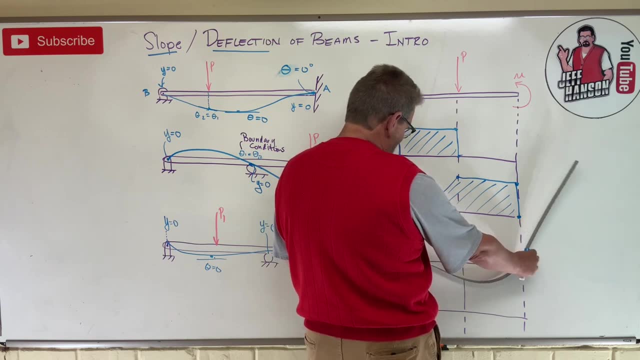 a fixed connection on this end and then it goes down. but on this end, over here, what, There's somebody that's like twisting on it which is going to make it go back up. so I might get something like that, okay, Because I'm twisting this over here. right, I'm twisting that, okay, So let's. 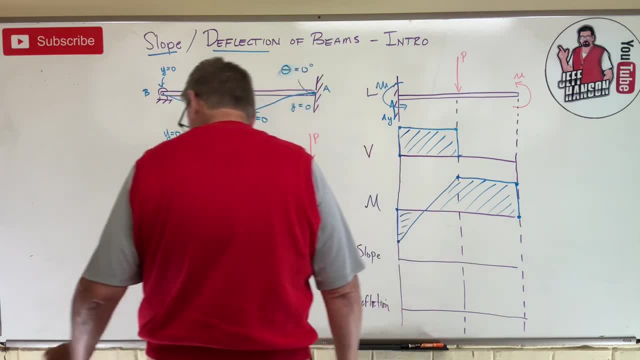 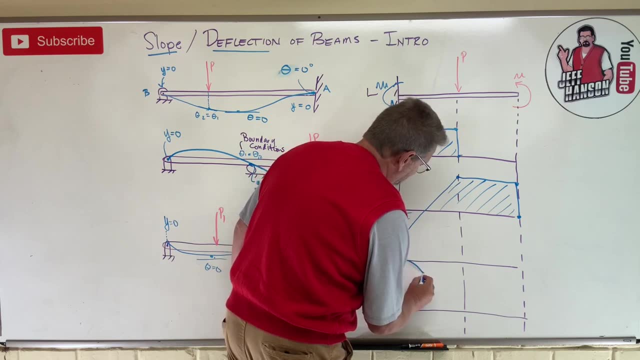 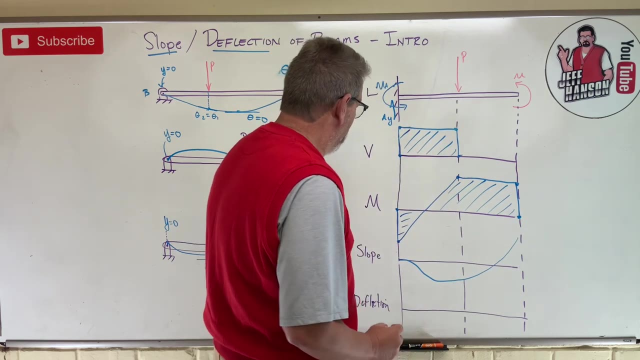 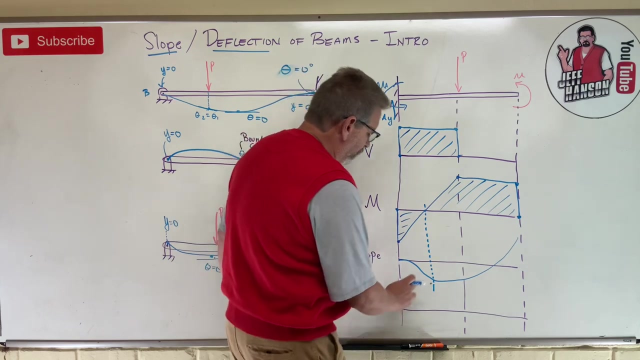 see if we can kind of sketch that kind of okay, So it's going to come out and then down and then back up to maybe like that: okay, Now, what did I draw there? okay, What happens here is right here, okay, Which I didn't draw, it super good, but I tried, I tried. 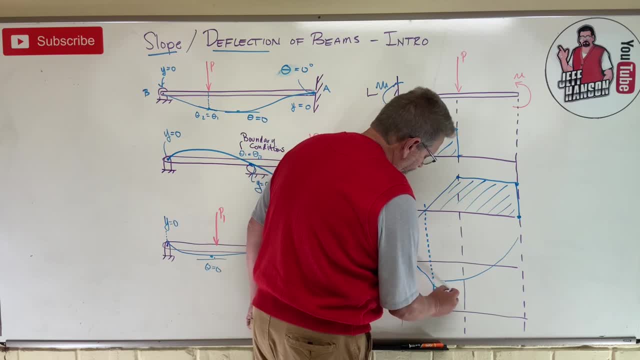 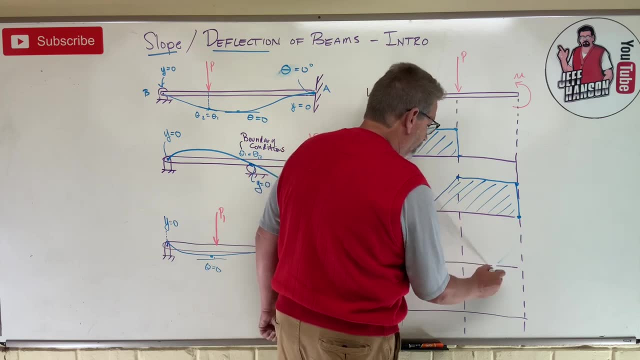 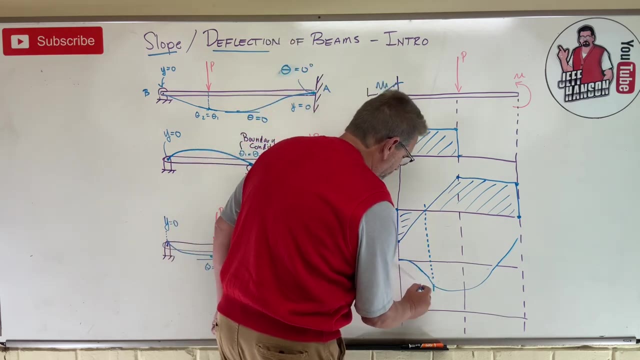 really hard, though. Okay, maybe that's a little bit better, Not really. That should be straighter, Okay. Anyway, what's going on there? okay, This guy right here is called the inflection point, And remember, that's where our moment went from negative to positive, right? 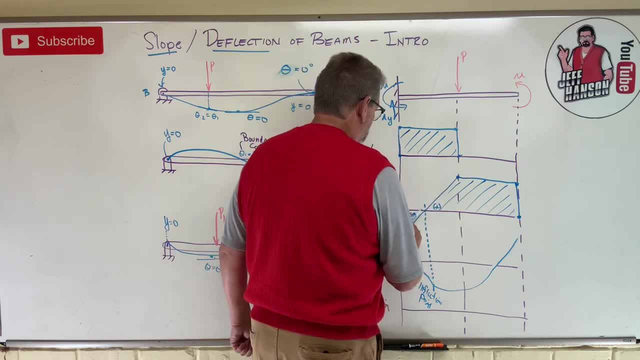 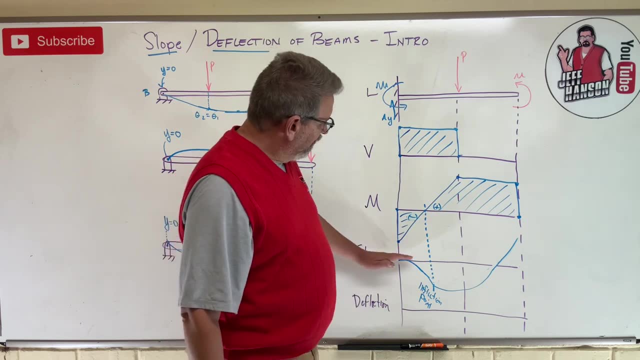 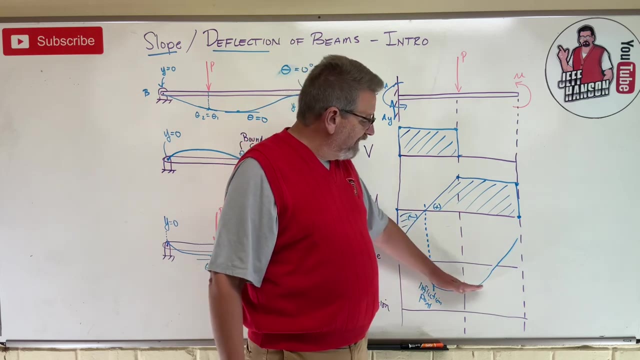 Whoops, I drew that exactly backwards, So we get an inflection point here. What is an inflection point? It's a point where the curve went from being concave down until that point and then the curve changed to concave up right. It changed the complete direction that the slope was headed. 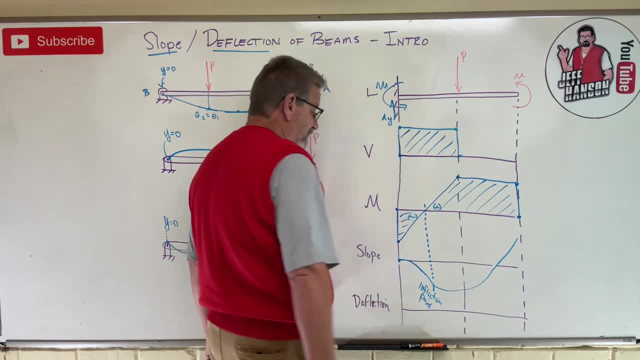 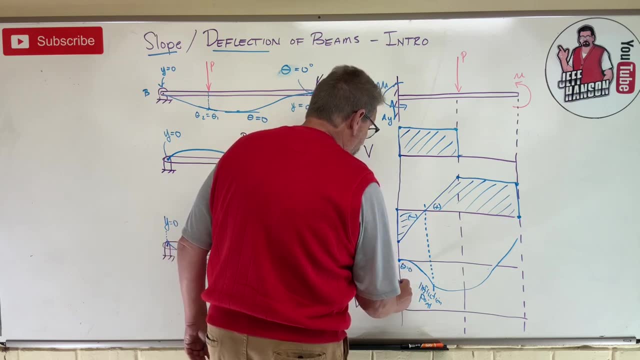 okay. So again, over here at the wall, we know that the deflection is zero, We know the slope is zero. So over here at the wall, we know that the theta equals to zero and we know, over here, y is going to equal zero. at that point Now the next video I'm going to